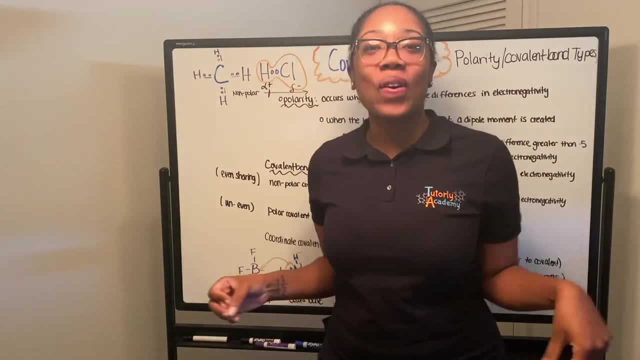 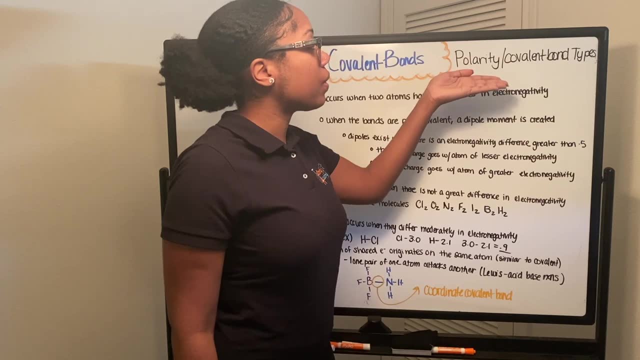 Hello there everyone, and welcome back to Tiddly Academy Tutorials. So today we are continuing our focus on covalent bonds, but we are specifically talking about what is polarity and what are the covalent bond types. All right, so we're going to go through this very quickly so you guys can. 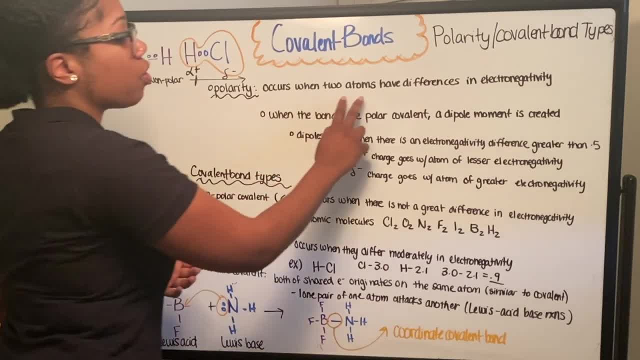 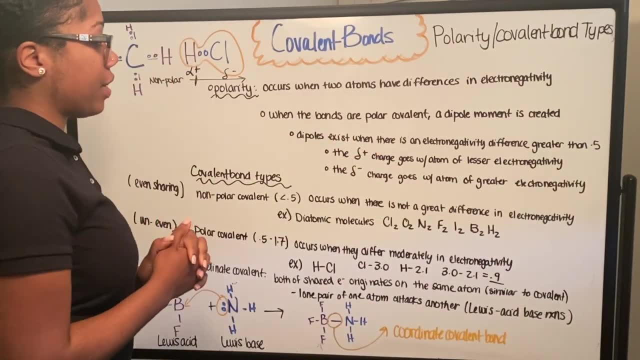 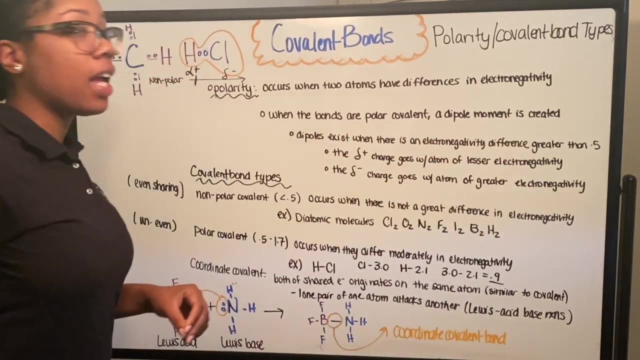 understand this. So polarity occurs when two atoms have differences in electronegativity. So these can be great differences or they can be minor differences. Now, when the bonds are polar, covalent, as you guys see here, a dipole moment is created. You're probably wondering. 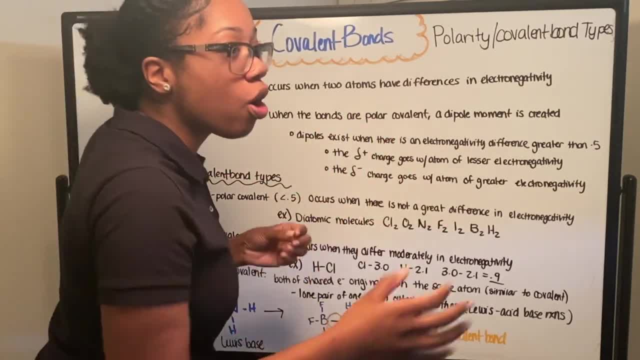 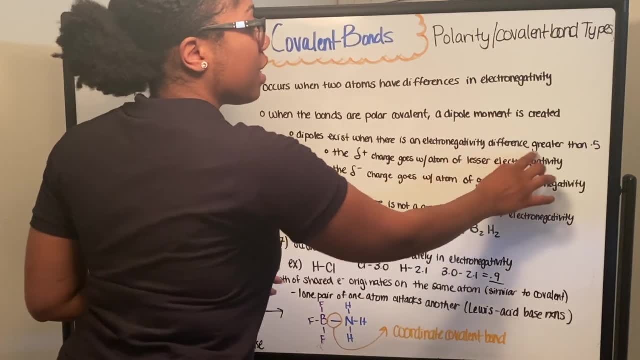 what is a dipole? A dipole exists, so dipoles meaning two poles. So there's a positive end and there's a negative end. So this exists when there is an electronegativity difference that is greater than 0.5.. Remember, we're talking about an electronegativity difference between two. 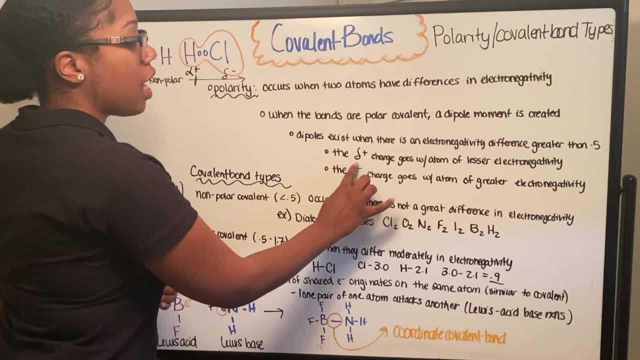 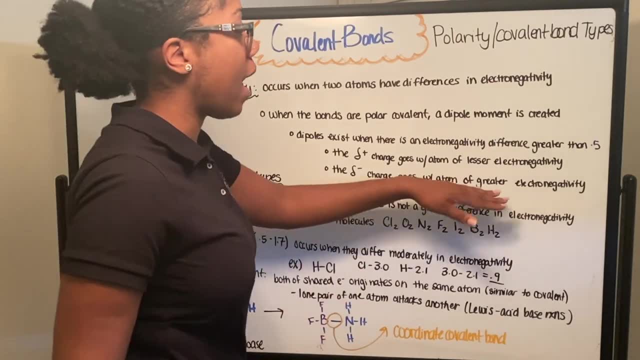 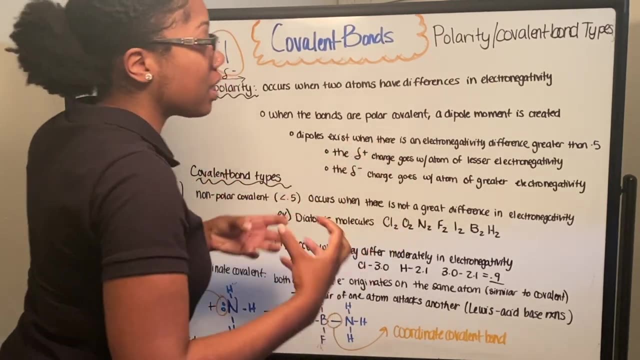 atoms. So the delta positive charge goes with the atom of lesser electronegativity and the delta negative charge goes with the atom of greater electronegativity. Or you can also look at it this way: The positive because poles begin to exist when. so let's look here. So you have chlorine. 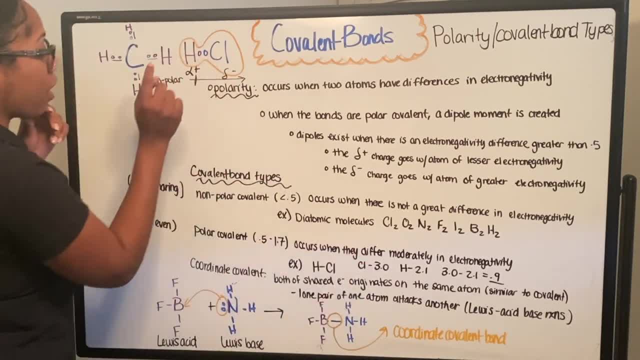 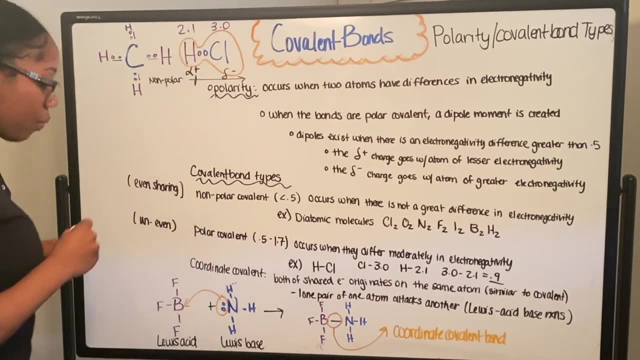 which has a electronegativity value of 3.0, right of three. And then you have hydrogen that has electronegativity value of 2.1.. So what it's saying here is that their overall electronegativity difference will be 0.9, which means it is a polar covalent bond. So why is that important? 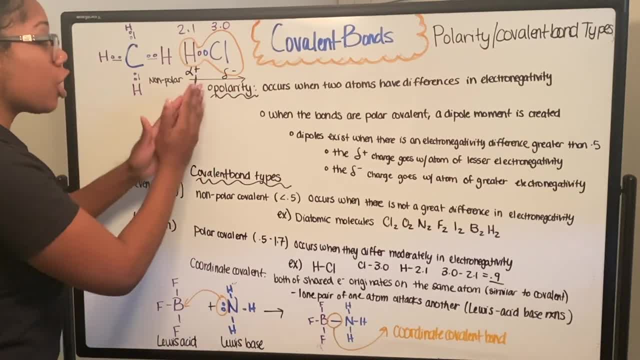 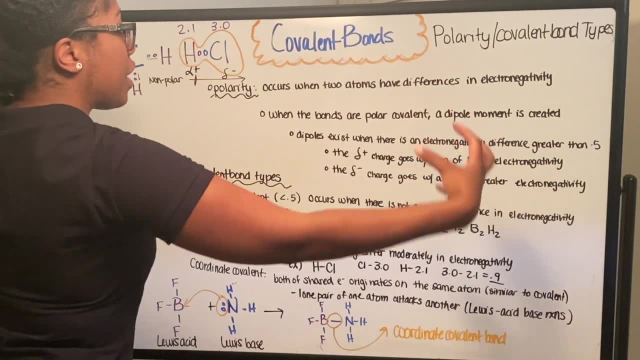 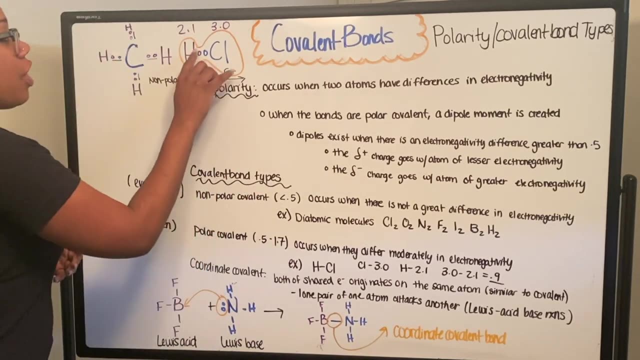 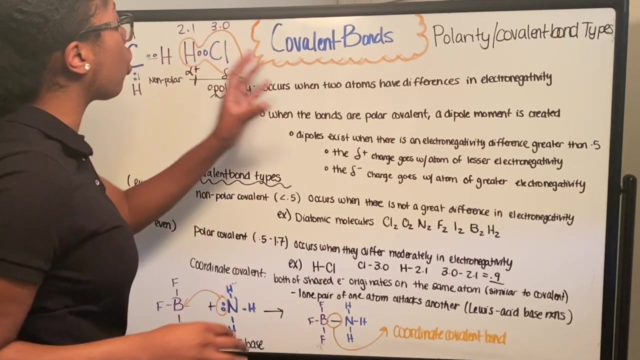 It's important because these two electrons that should be equally shared between hydrogen and chlorine, because of this greater difference in electronegativity- You guys see this orange thing that I drew here. That is the electron density. These two electrons are going to spend majority of their time circulating or surrounding chlorine. 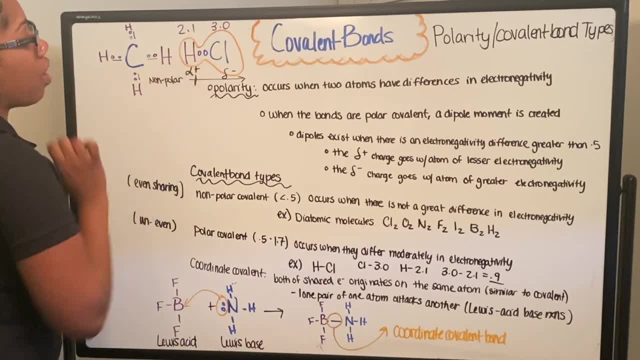 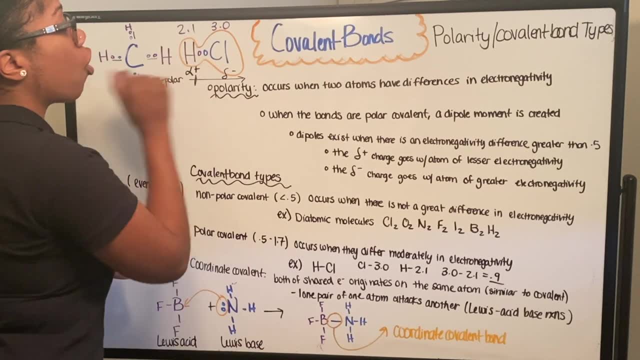 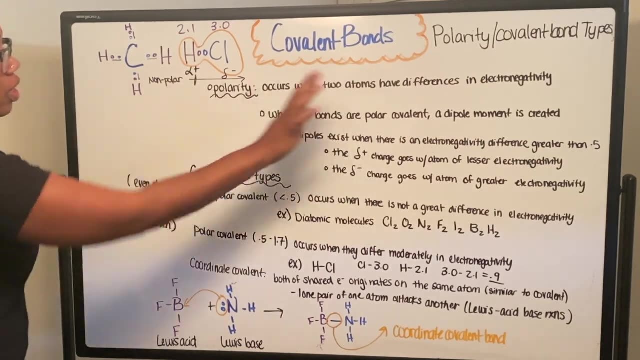 whereas it's not going to be as much electron density here. That is why the hydrogen gets the partial positive or delta positive, and chlorine gets the delta negative. Now, this thing here is the dipole, where you start at the positive but it directs towards the negative, because that's where 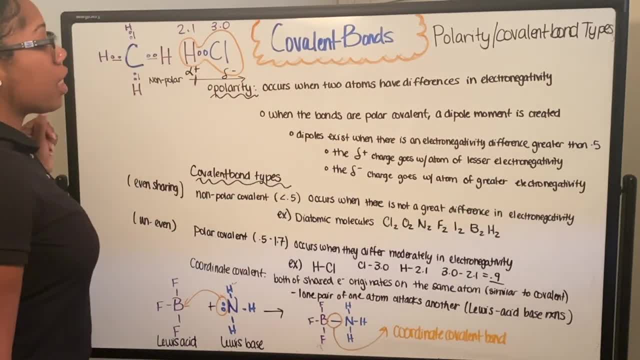 majority of the energy or the electron density is going to be. So that's why the hydrogen gets. the majority of the density is going towards Okay. so now that brings us to the different covalent bond types. Now, in non-polar covalent there's an even sharing. So here this is a covalent bond because 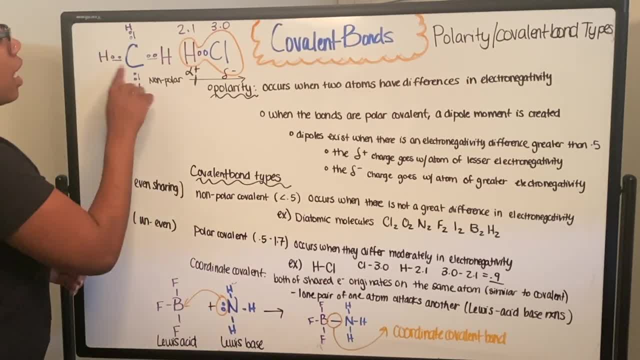 they're sharing, but it's non-polar because if I remember correctly, I think I know hydrogen is 2.1, but I think chlorine is like 2.4 or something like that. They're really close in electronegativity value. So when there is not a great difference in electronegativity value, they're not going to. 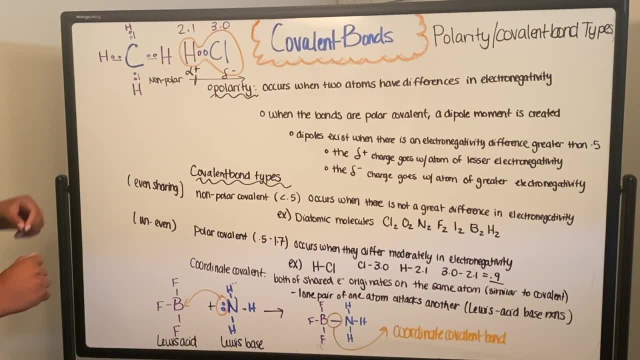 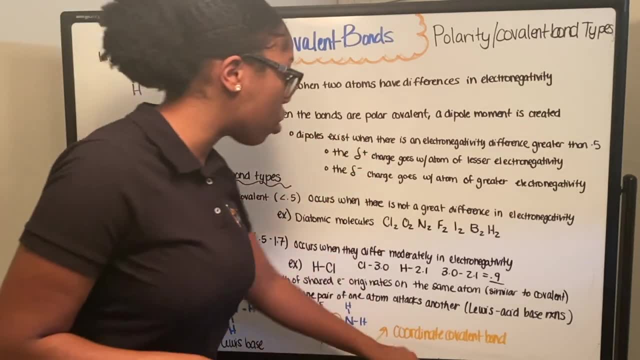 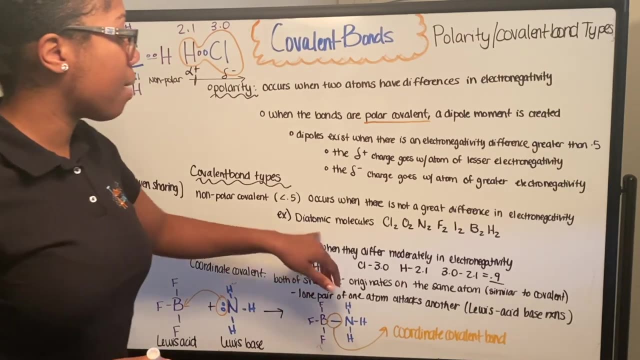 be the same. So we get these non-polar covalent bonds. So, as you guys notice, there's no dipole moment created here, because dipoles are only created when it is polar covalent. Okay, so for non-polar covalent, for example, you have diatomic molecules, So you have chlorine oxygen. 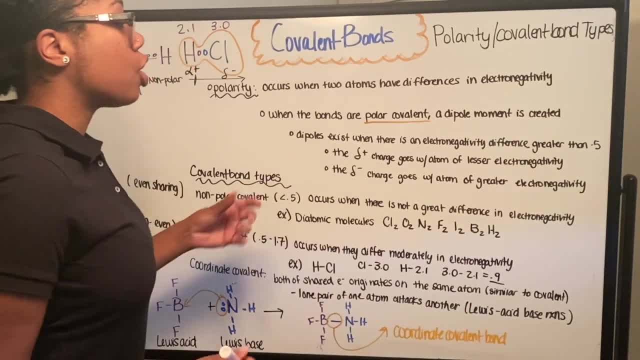 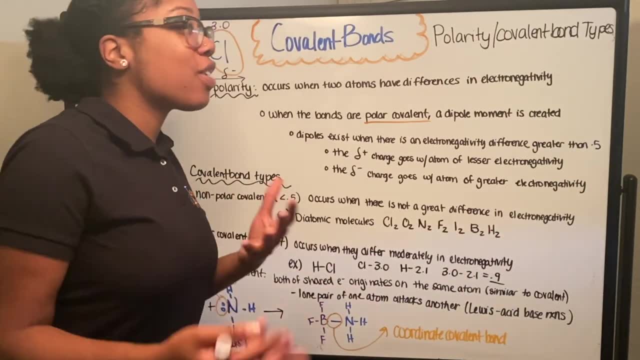 nitrogen, fluorine, iodine, bromine and hydrogen. So when you have two of these, two of the same atoms together, it's like subtracting itself. 2.1 minus 2.1 is zero. So there is no difference in electronegativity value. therefore there is an. 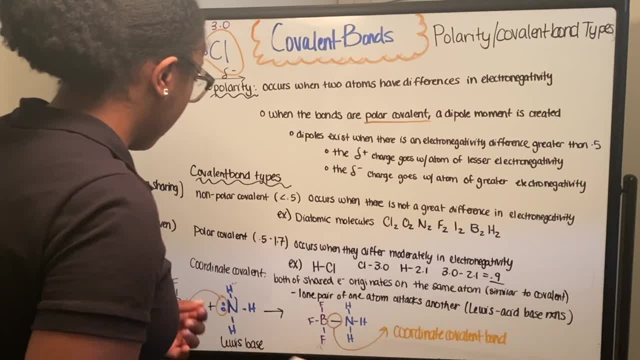 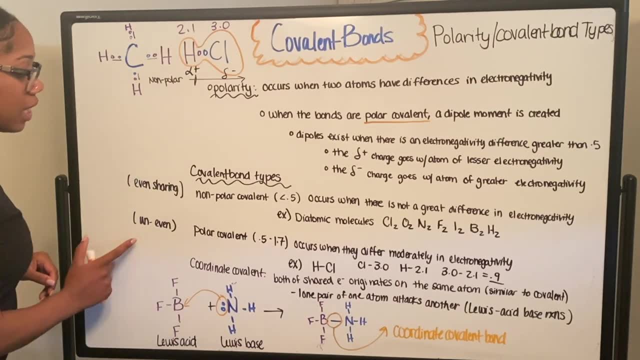 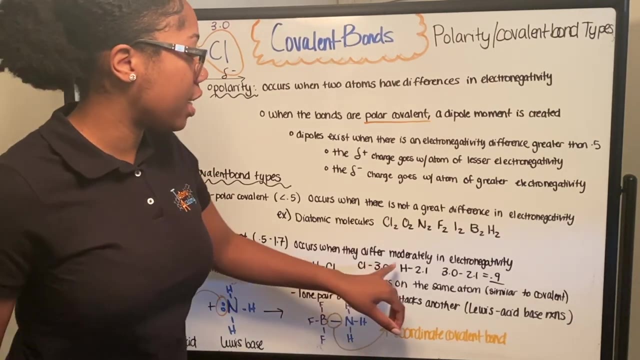 equal sharing or an even sharing, I should say, of electrons Now with polar covalent. as you guys saw here, with HCl or hydrochloric acid, there is an uneven sharing of these electrons. Okay, so it occurs when they differ moderately in electronegativity. So there is a certain value. So for non-polar covalent it's when it's less than 0.5.. For polar covalent, it's when it's 0.5 to 1.7.. Okay, so then I just wrote out the numbers that go along with this example up here. Now the last type of covalent bond types that we 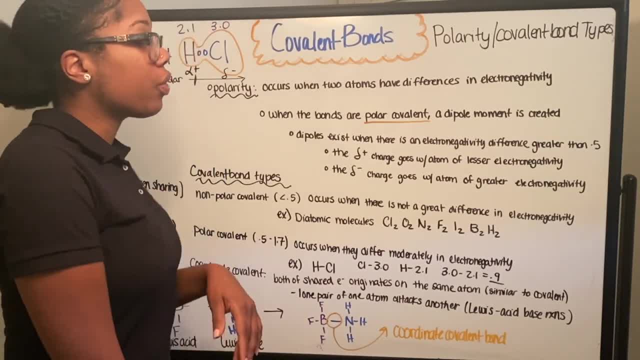 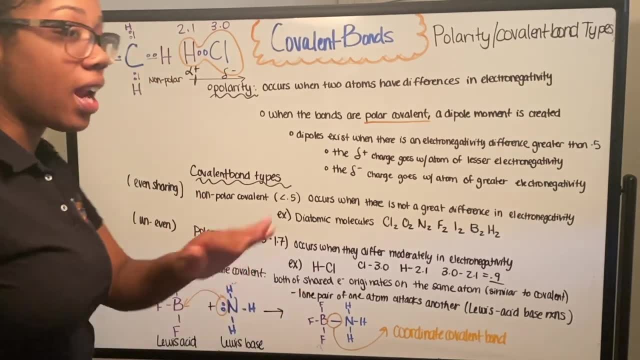 have are coordinate covalent bonds. Now, in general chemistry you won't encounter these as much as you will in organic chemistry, but it is, or in high school chemistry even. But what is a coordinate covalent bond? So it's when there's two of these electrons. So it's when there's two of these electrons. 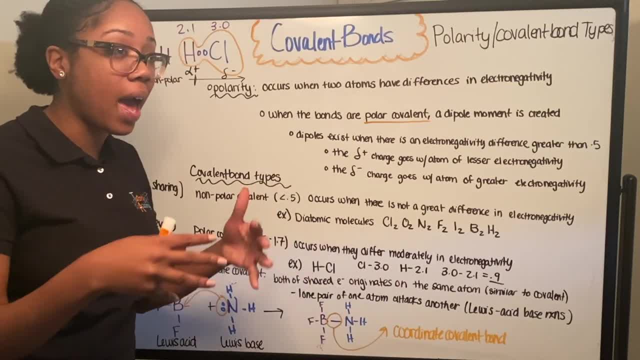 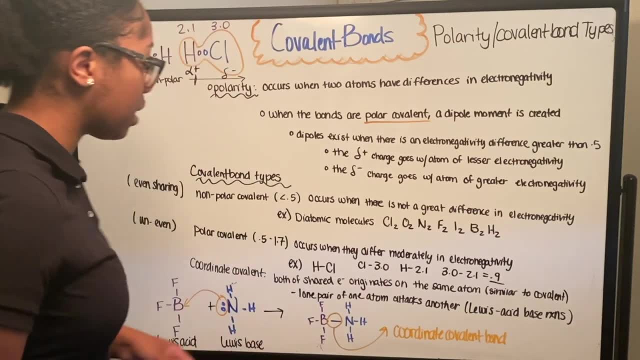 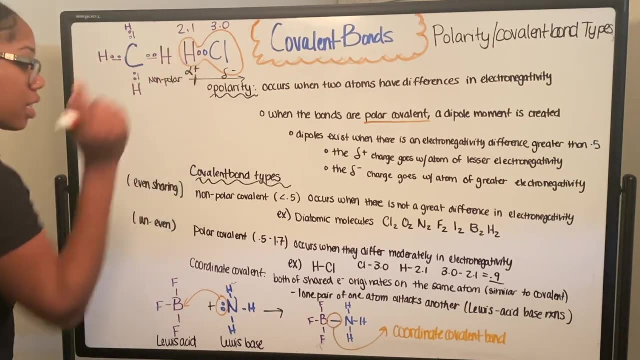 that are going to be shared between two atoms, but they originate off of one atom. However, the reason why I have similar to covalent is, if you guys look here, you can't tell the difference between this coordinate covalent bond and this covalent bond or this covalent bond, right? So it's just. 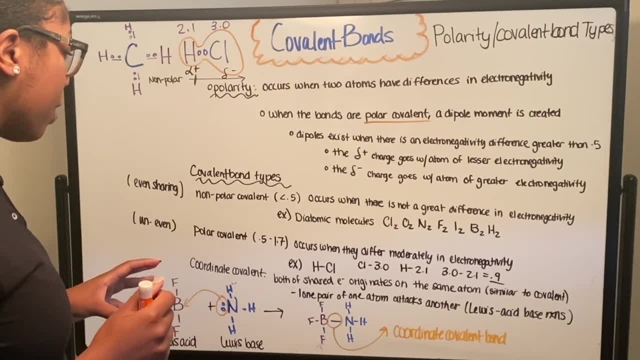 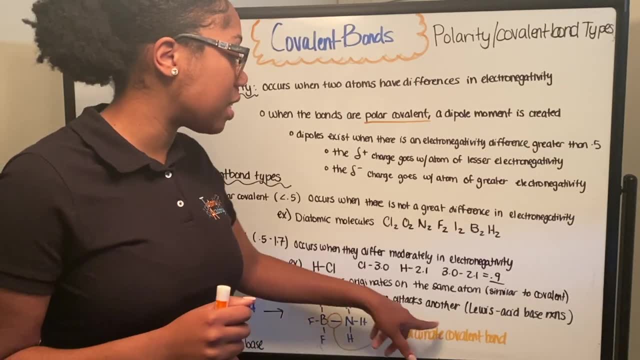 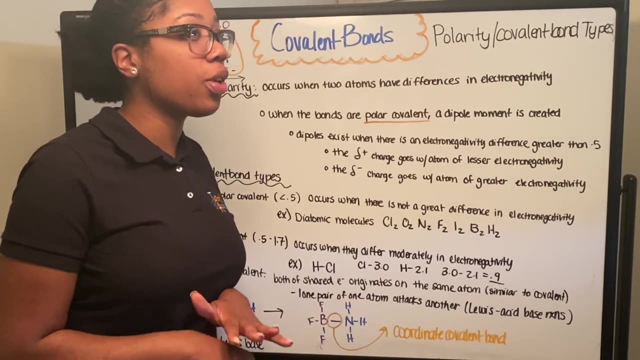 really important that we kind of understand this, okay. So let's look at um. so yes, essentially what happens is the lone pair of one atom attacks another, So you have the Lewis acid base reactions. Those are the prime examples. The reason why I say you guys may not encounter that. I think you will. 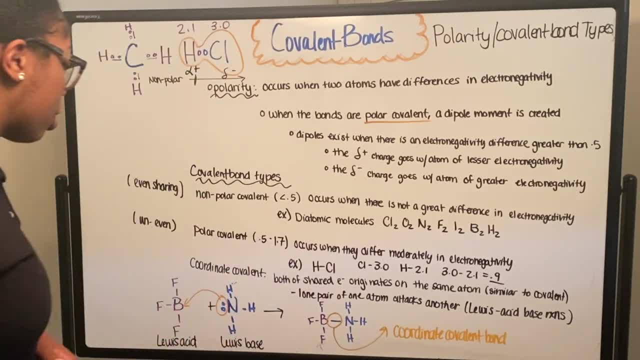 encounter it in general chemistry but not in high school level chemistry, So you guys can just skip past this portion. But if you guys look here, this is the Lewis acid. Why is it an acid? Acids are known to need electrons. Acids are known to have to be the um acceptor of electrons, right A Lewis. 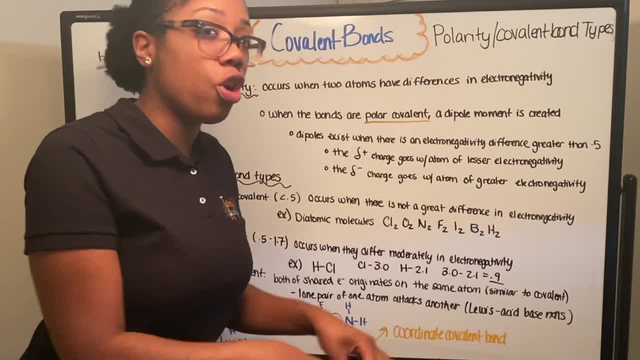 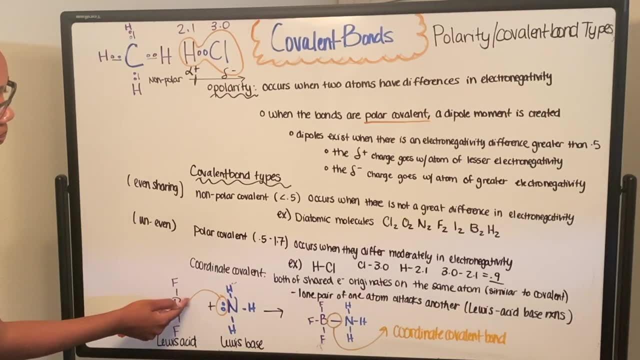 base. Bases are known to be these electrons. So if you look here you can see that the Lewis acid is the electron donor, The ones that are donating the electrons. As you see here there's nothing on this boron atom, But as you look here on nitrogen there are two electrons that are here. 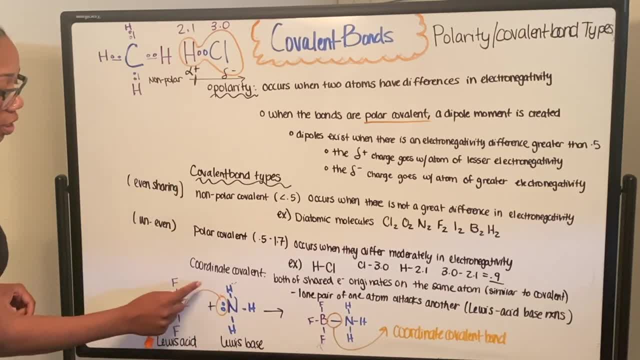 Two lone pairs. I mean one lone pair that is ready to be shared with this. So this nitrogen or this ammonia atom, it donates its two electrons to this boron to form what we call a coordinate covalent bond. So if you guys look here you can see that the Lewis acid is the electron donor. So if you 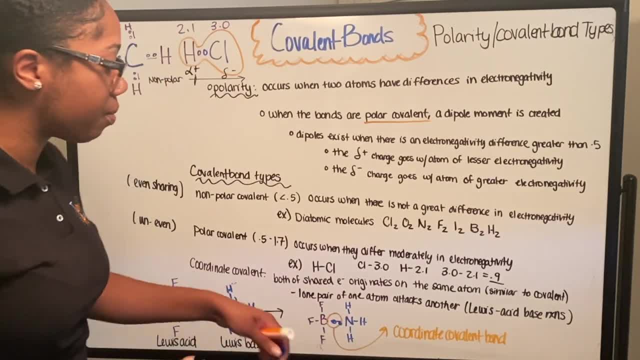 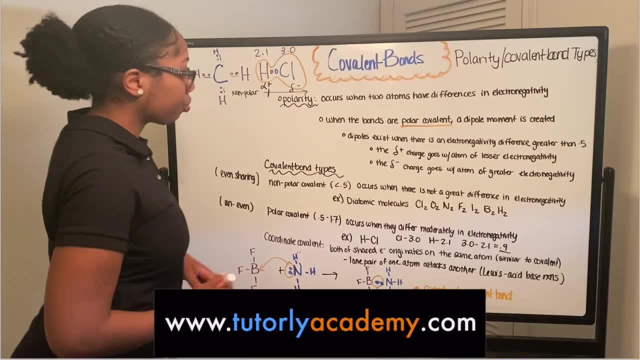 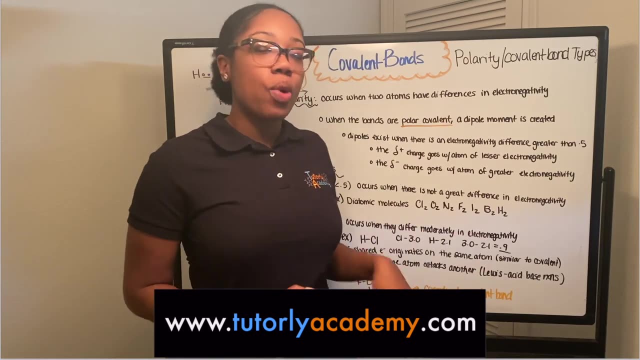 guys look here, you can see that the Lewis acid is the electron donor. So if you guys look here, you can dentro one particular molecule which is Ammonia. So, overall, this is a brief overview of what polarity is and the covalent bond types. We will go more into detail about, I believe, this Lewis acid. 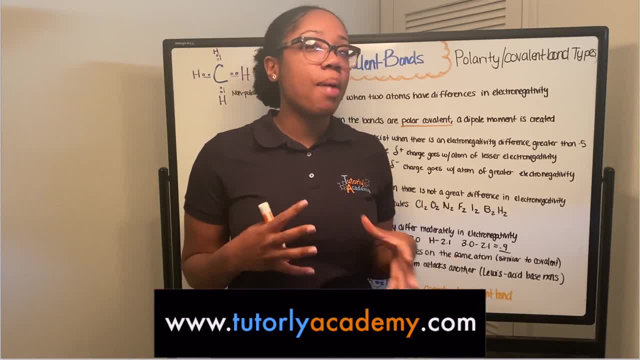 structures that we're going to start talking about next So that you guys can make a lot more sense of these things. But we're going to talk about those things next week. We are going to do like a quick. We are going to do like a quick brush: Pour into the sotto voile cell, Because you guys know all of was a aroma And you guys twelve little placenta".